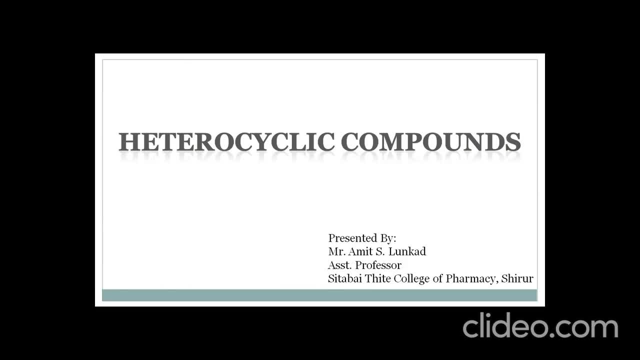 are having many uses. Hi, I am Amit Lunkard. In this video we discuss about the meaning of heterocyclic compounds and nomenclature of these heterocyclic compounds. Let's begin with the meaning of heterocyclic compound. A heterocyclic compound is the cyclic compound. 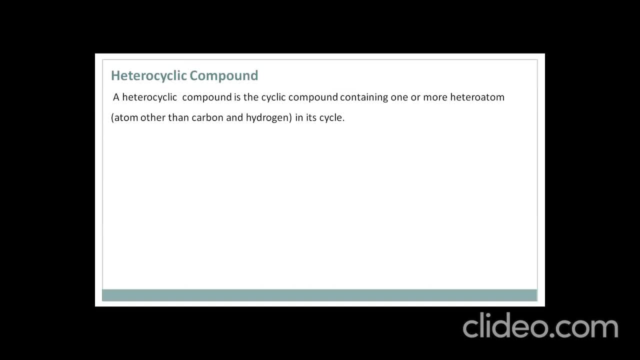 containing one or more heteroatom in its cycle. Heteroatom means an atom other than carbon and hydrogen. The most common heteroatom present are nitrogen, oxygen, sulphur. Here is the structure of benzene ring, And if you see this, it just. 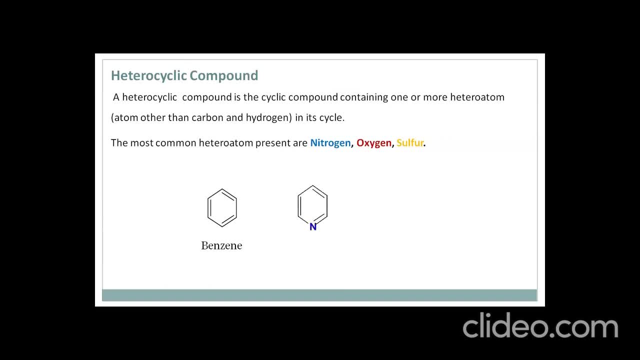 having a carbon and hydrogen, But in this structure, with carbon hydrogen it having a nitrogen, And this nitrogen we call as a heteroatom. So this compound is called as a heterocyclic compound And this is the structure of pyridine. So these are about the meaning. 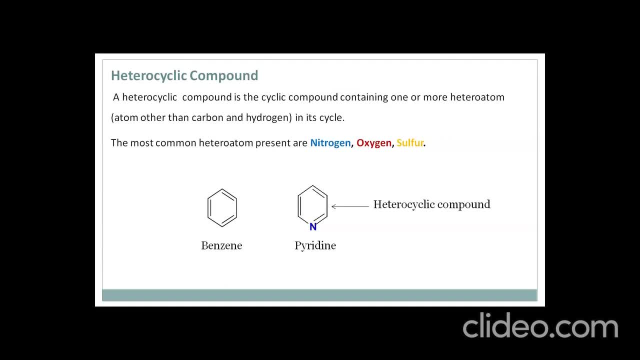 of heterocyclic compounds. Hi, I am Amit Lunkard. In this video we discuss about heterocyclic compound, heteroatom, which are present in a cyclic ring with carbon and hydrogen. Now about the nomenclature which are given to this heterocyclic compound: The heterocycles. 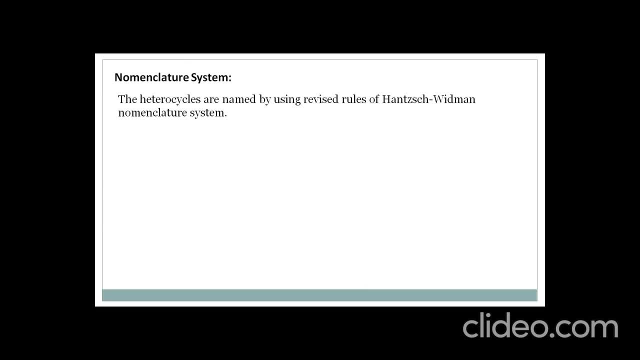 are named by using revised rules of Hans Widmann nomenclature system. Here we discuss about the monocyclic containing single heteroatom And we use some rules for this. First is there is a heterocyclic system is named by combining one or more prefixes for the heteroatoms with the stem. So first is about combination. 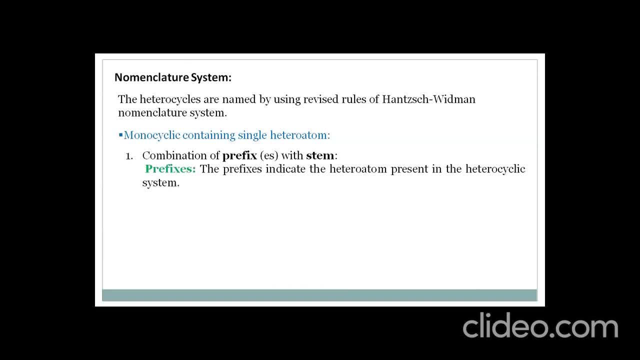 of these prefixes with stem. So what is prefix? The prefixes indicate the heteroatom present in the heterocyclic system And stem means the, which is a heterocyclic compound. So it is used to indicate the size of the ring and the saturation or unsaturation in the 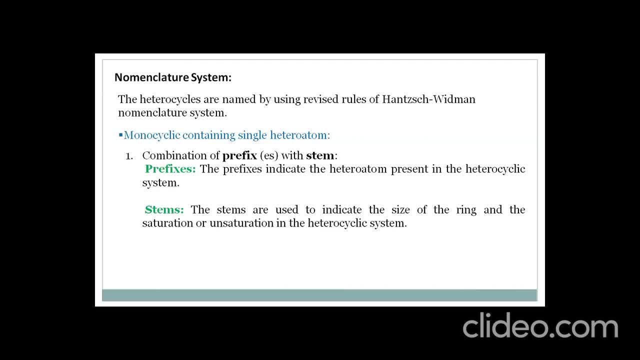 heterocyclic system. So stem means this, indicate the size of ring, means whether it is a three member ring, four member, five member, six member, six member and so on. So we combine this prefix and stem to form a name to this heterocyclic ring. So first is about the 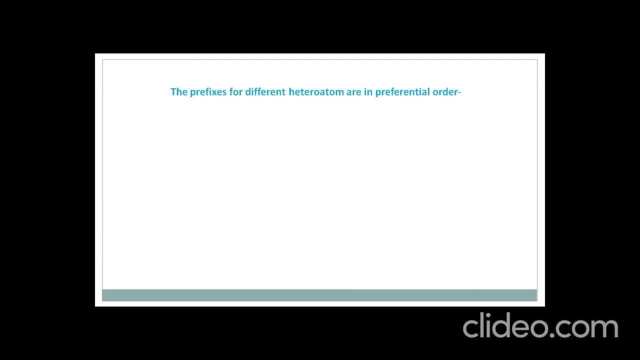 prefix stem. So first is about the prefix stem. So first is about the prefix stem. First is about the prefix stem. So first we have the two prefixes for the different heteroatoms, which are in preferential order. So here is the heteroatom like oxygen, sulfur. 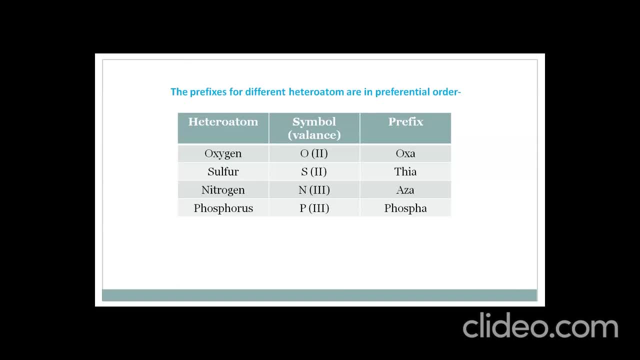 nitrogen and phosphorus. So which are the prefixes we use for this? So, if your ring having oxygen, so we which having a symbol O and it having a valency of 2. So we use prefix oxa. 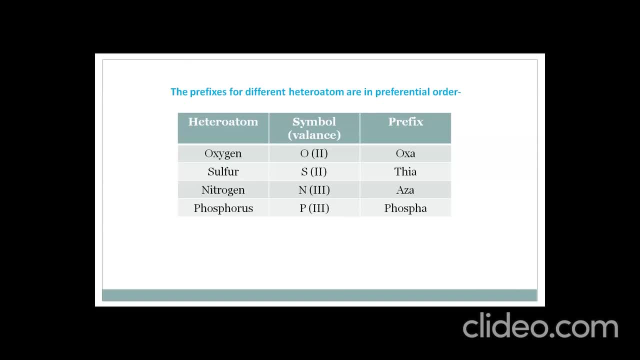 the symbol is S and it having a valency 2, we use prefix Thaya. For Nitrogen symbol is N and which having a 3 valency, and we use Aza as a prefix, And for Phosphorus the symbol is P. 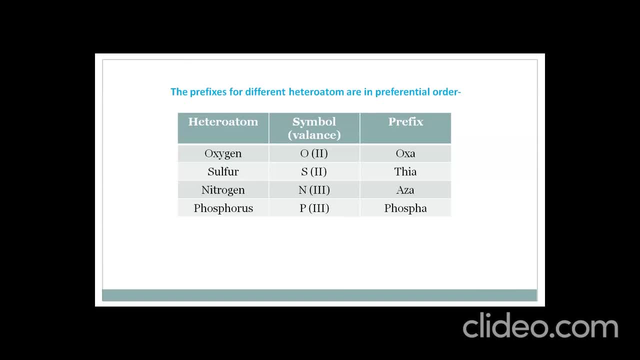 it having a valency of 3, and we use the prefix Phosphor, So you have to remember this prefix for the heteroatom, for Oxygen, Sulphur, Nitrogen and Phosphorus- Most of the heterocyclic compounds. 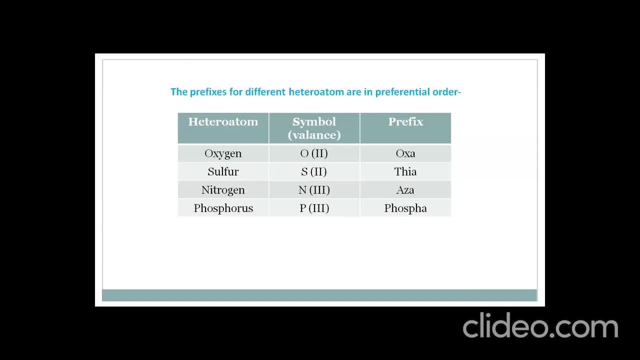 having a Oxygen, Sulphur and Nitrogen. So remember for Oxygen, Oxa for Sulphur, Thaya for Nitrogen, Aza. Now here we use stems for 3 to 10 member heterocyclic compound and 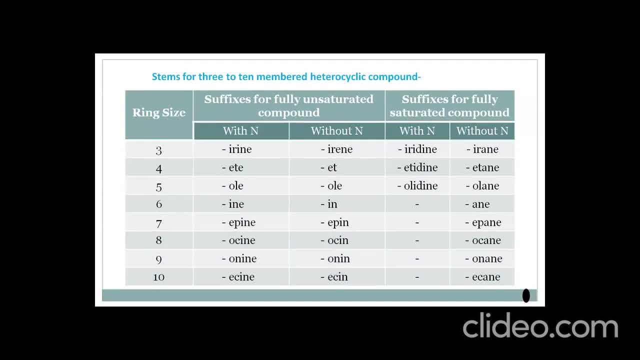 whether these are saturated or unsaturated, whether they contains Nitrogen or without Nitrogen, Like here: if the ring size is 3,, then if it is unsaturated one and with Nitrogen, then we use the stem I, R, I, N, E, Iren, and if it is unsaturated, 3 member ring without Nitrogen. 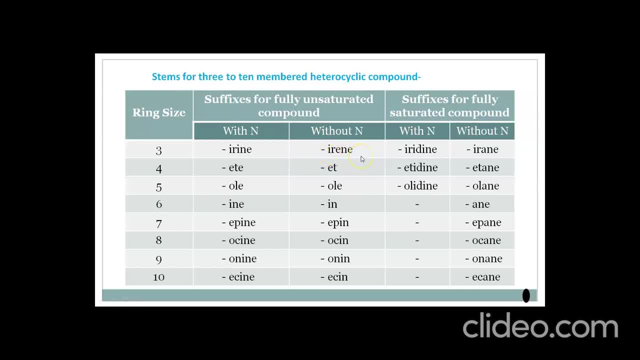 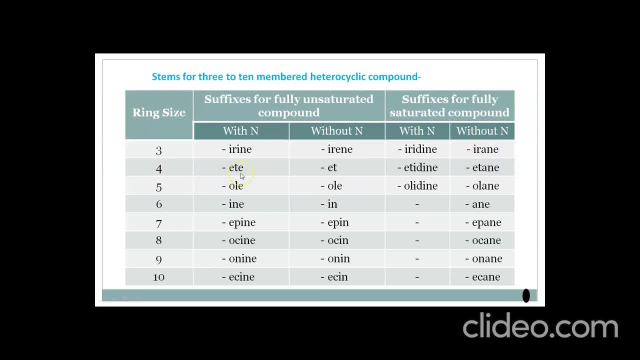 with Nitrogen, E T E stem we use and unsaturated 4 member ring without Nitrogen stem is E T, But if the 4 member ring which is completely saturated with Nitrogen, then we use stem E T D. 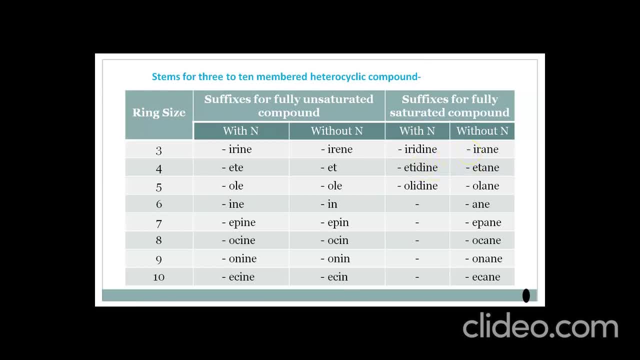 example, by注意 list stem OLE, otherwise symbol 12.. City is saturated with Nitrogen E, T D tap I Iren to say 14, and without Nitrogen 4 member ring saturated 1, we use the stem E10.. 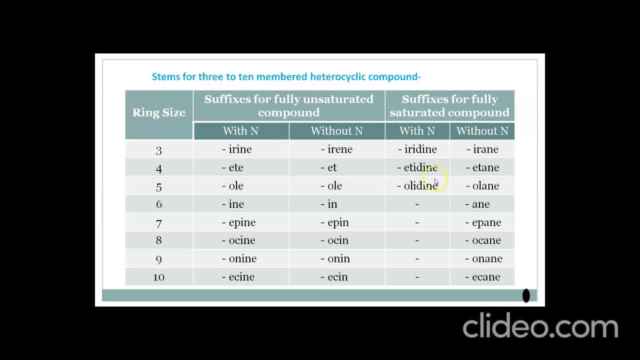 Like if it is a 5 member ring which is completely unsaturated and with Nitrogen, then we use stem OLE Both for without nitrogen, the 5 member ring also, we use stem OLE. But if this 5 member ring which is completely saturated, 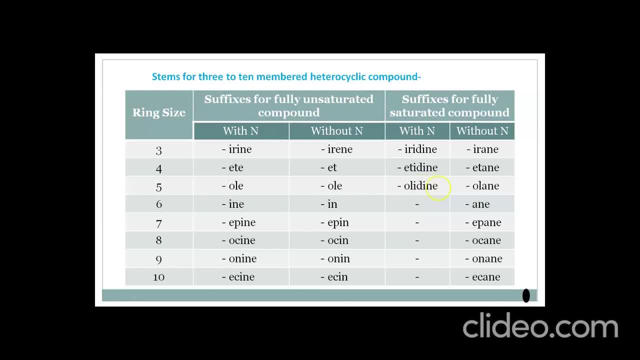 I will just add this name: Stem OLE. I frolicated 2. Stem OLE with Nitrogen, then we use Olidine and without Nitrogen, 5 member saturated ring, we use the same Olane Like for 6 member ring. INE IN for unsaturated compound for the 6 member ring, if it is. 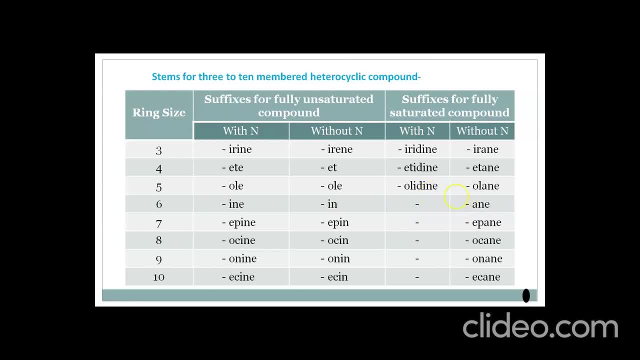 saturated without Nitrogen, we use the same ANE and no more any stem we use for the with Nitrogen. So these are the according to ring size and the nature of the ring: whether saturated and unsaturated, we use this same. 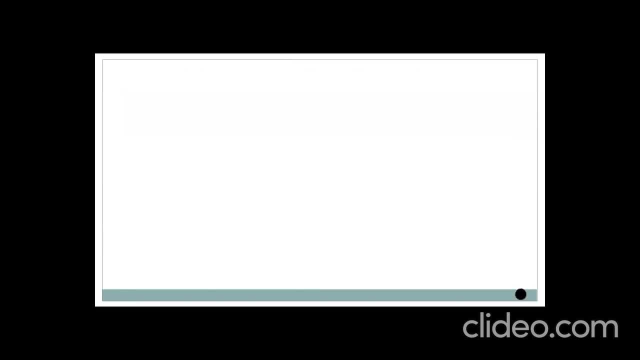 So you have to remember this, So to know this. we have some examples, like: here is the: this hetero cyclic ring, as it contains a Carbon Hydrogen and with this, Oxygen, So Oxygen is a heteroatom, So as it is having a Oxygen, 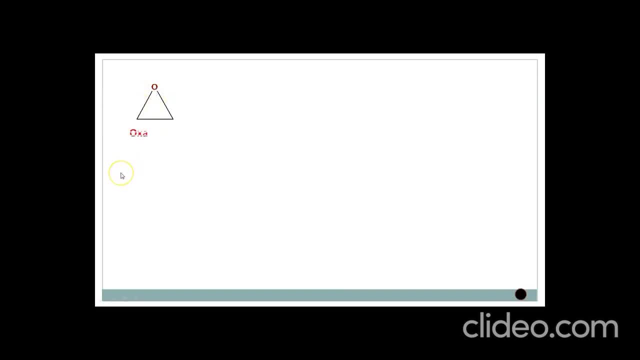 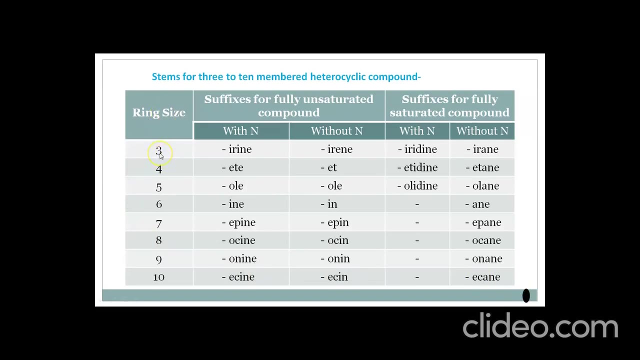 So for Oxygen We use the prefix Oxa. Now here it is a completely saturated ring and without Nitrogen. So which stem we use? So look, here it is a 3 member, ring size is 3 and which is completely saturated one. 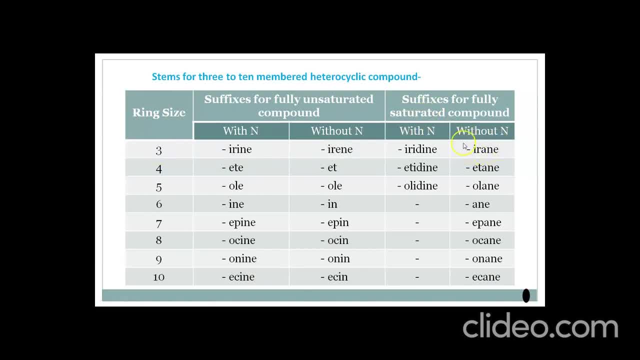 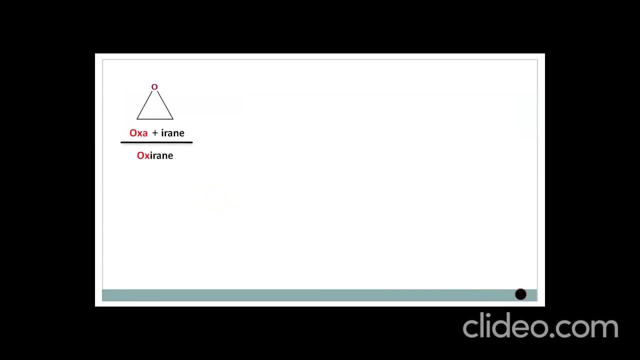 and without Nitrogen. So we we use the same Iron, So just give it plus Iron. So name of the ring is Oxa, Oxa, Oxa. So name of this compound or name of this hetero cyclic ring is Oxirane. 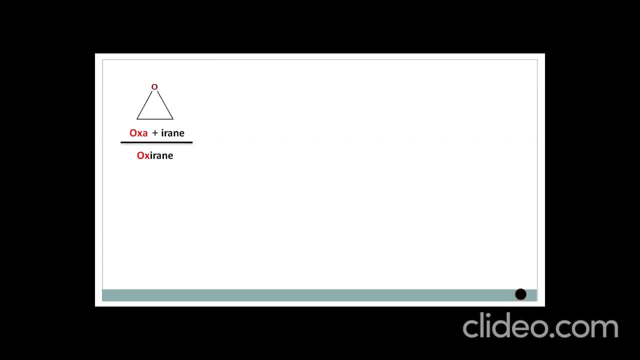 To know much more about this. we take second example. like here, it is a 3 member ring, but having a heteroatom, Nitrogen. For Nitrogen we use the prefix Aza. So which stem we use for this? 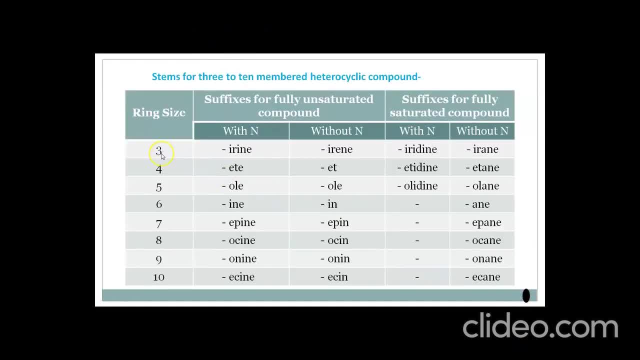 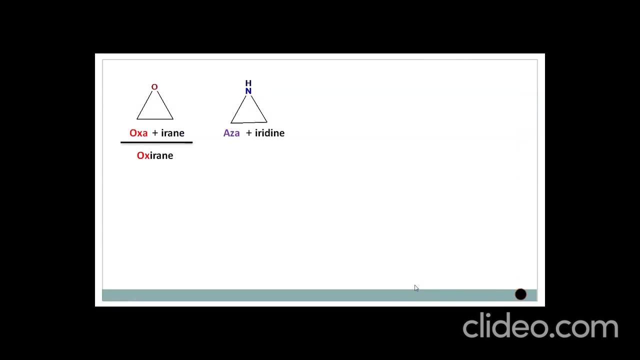 So here it is, a ring size is 3.. It is completely saturated, Saturated one and with Nitrogen. So with Nitrogen saturated ring we use the same Iridine. So just put it So plus Iridine. So name of the compound is Aziridine. 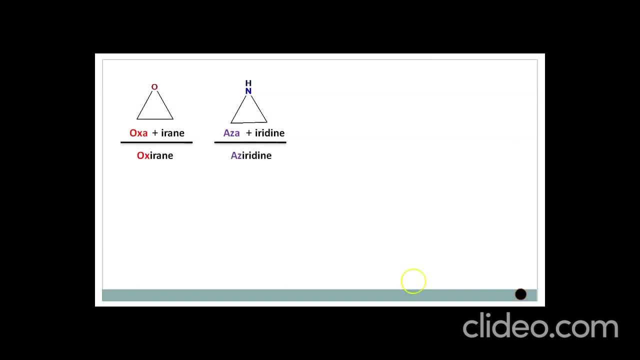 So, with these two example, you will also know that here is the Oxa, but here is the A is drop, Here is Aza, but A is drop. So while giving this or combining this, You have to remember, if the stem begins with the oval, the terminal letter A of the prefix. 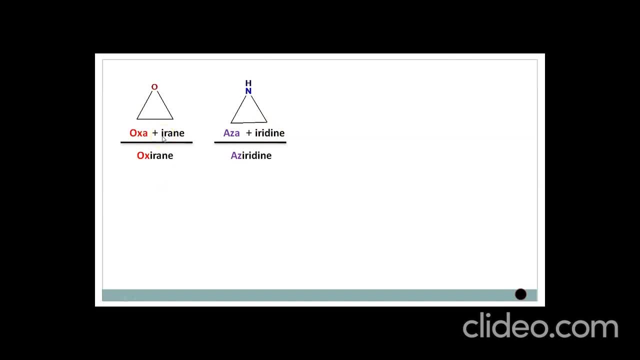 is drop. Yes, Here the stem is starting with oval I So we drop this A of the prefix and that's why the name is Oxirane. Oxirane, Same for this Aziridine. We drop this A of the prefix because the stem is starting with oval. 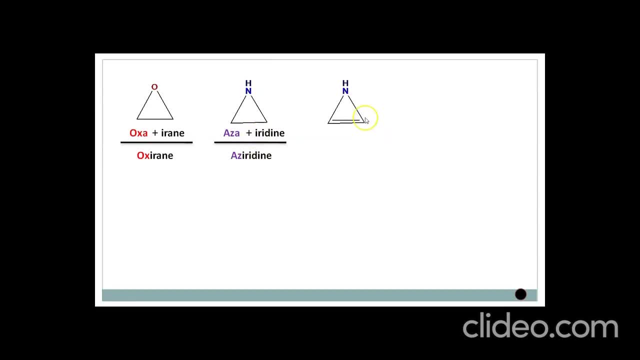 Now, next example is now here. it is the 3 member ring size is 3 and it is unsaturated one and it contains Nitrogen. Yes, Obvious, for Nitrogen heteroatom we use Aza. Then for which unsaturated 3 ring size, which stem we use? so look here the ring size is: 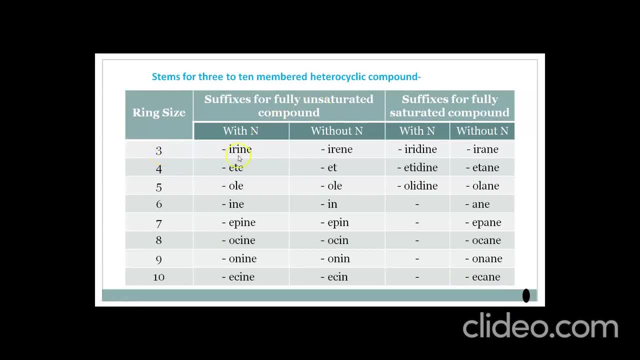 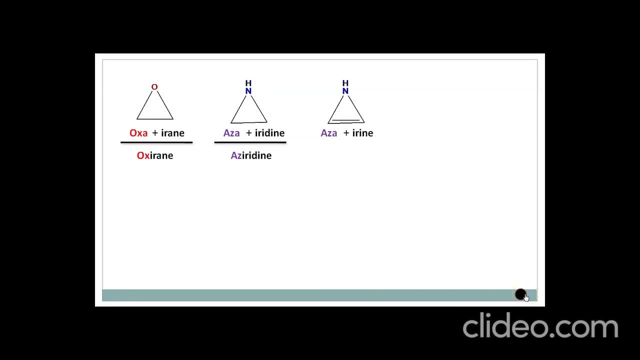 3. It is unsaturated one with Nitrogen, So we use Iriane Irene, So just put it here plus Irene, So name is yes, it is. stem is started with the oval, So you have to drop this A, So name is Azirine. 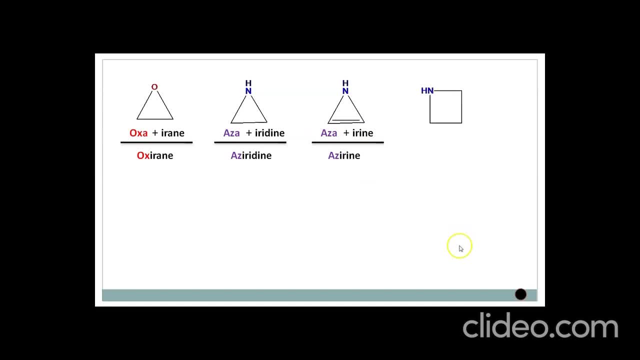 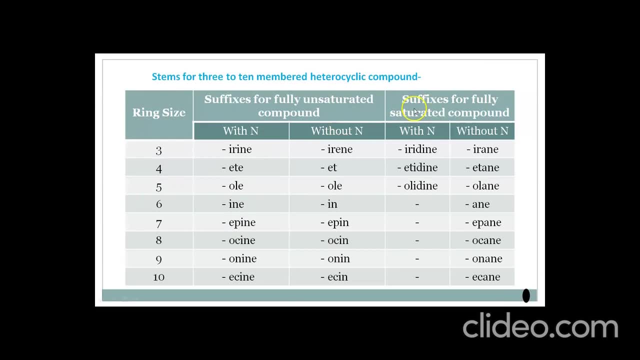 Same for the next one. It is a 4 member ring which is completely saturated one. So look, here it is a 4 member. Now it is saturated one and with Nitrogen, So it is Ethylene. You have to use this name: Ethylene. 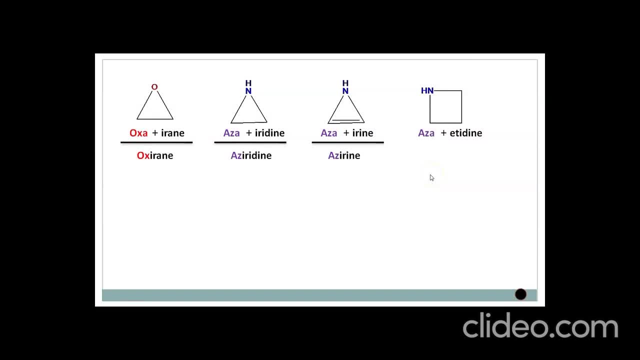 So for Nitrogen, Aza plus Ethylene, So name is Azitidine. Next is here. it is a ring size is 5 and having heteroatom Oxygen, So for heteroatom Oxygen, Oxa. Now here it is a 5 member ring. 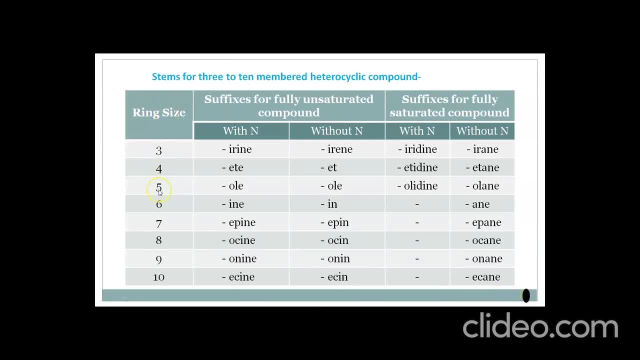 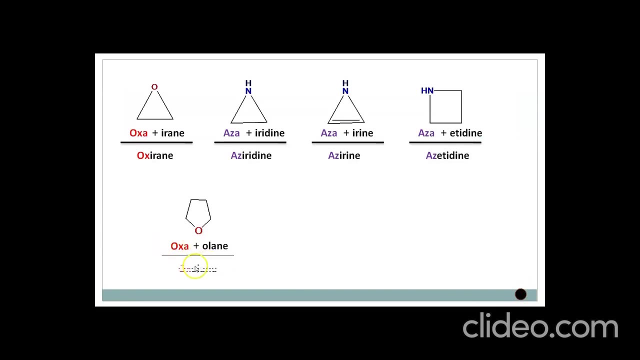 So it is a 5 member. Our ring size is 5 and it is a completely saturated one without Nitrogen, So O-L-A-N-E, So you have to plus Olane, So the name is Oxalane. Next is the here the 1,, 2,, 3,, 4, 5, 6, 7, ring size is 7 and it is unsaturated one with. 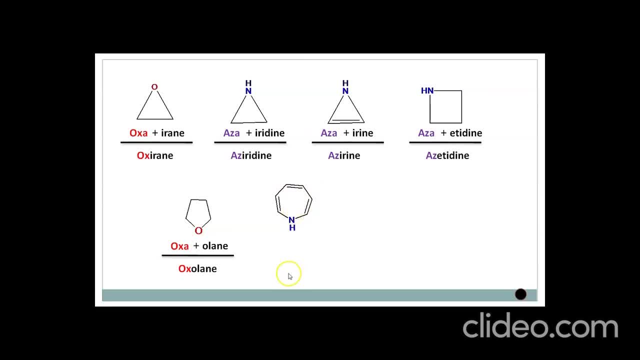 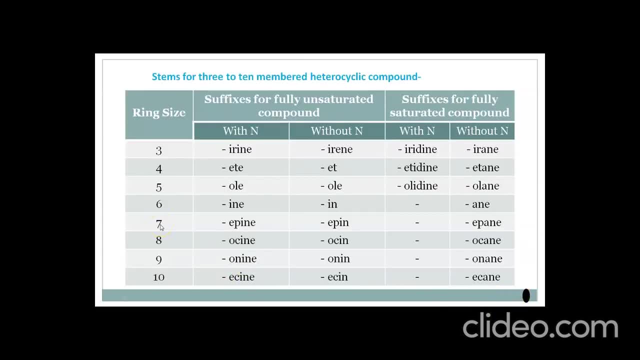 Nitrogen, For Nitrogen heteroatom Oxalane. Ok, Put the prefix Aza. Now here we see it is a ring size is 7 and which is unsaturated one with Nitrogen, So we use the same Epine. 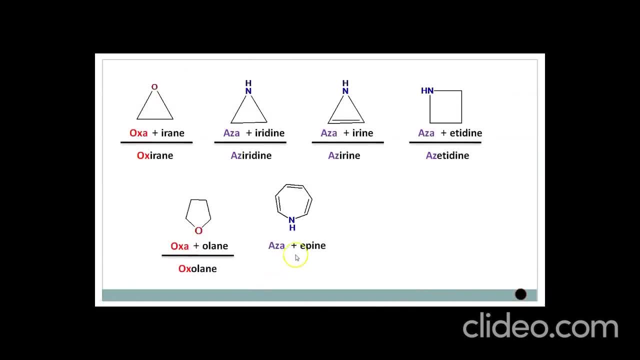 So just write it and it starts with the same. it starts with the O-L, So drop this A, So name is Azepine. Same for here. it is Oxygen, So it is O-L-A-N-E. Ok, So these are the example. 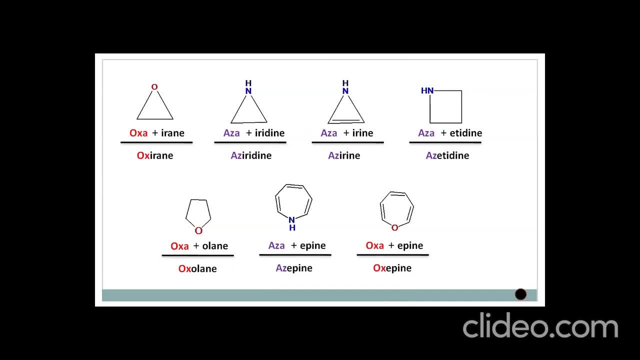 Here we use the combination of prefix with stem and we have given the name for that particular heterocyclic ring. Moving to the next point, which is the presence of identical heteroatoms, means multiplicity of heteroatom. So your heterocyclic ring contains more identical heteroatom. 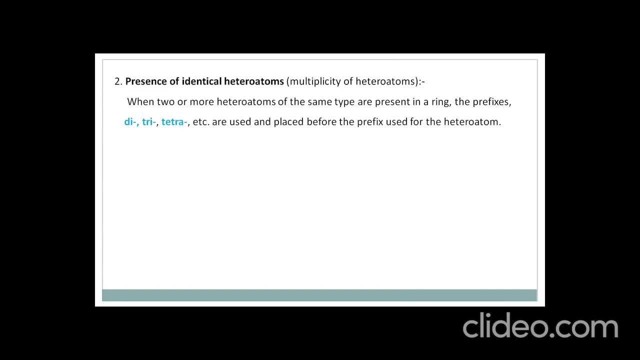 So what to do? So when two or more heteroatoms of the same type are present in a ring, the prefixes di, tri, tetra, etc. are used and placed before the prefix used for the heteroatom. Like di means it indicates the two heteroatoms are present which are identical. 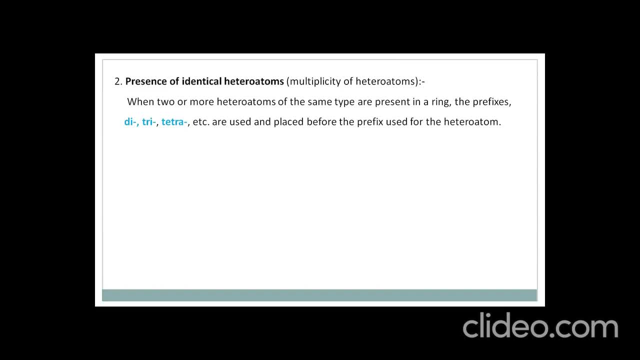 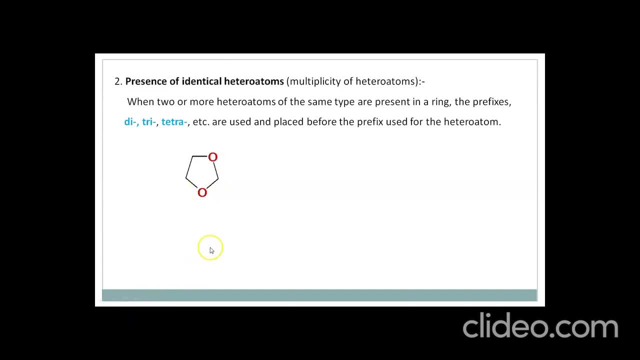 are oxygen. Just now we have used the. we have seen one example in which the five member ring, which is saturated and with oxygen, the name we use is an oxalon, But here there is the presence of two oxygen or two heteroatoms. 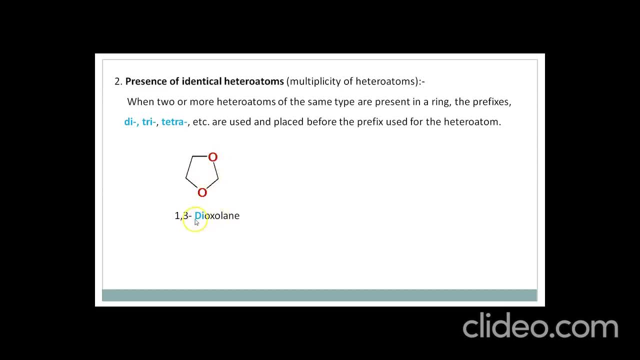 So we use the di Now, before that we use this prefix di. So it is the dioxalon, and here we have given the one. three means. it indicates the numbering to which they are present. This point we discuss later on. Let's move with the second example. 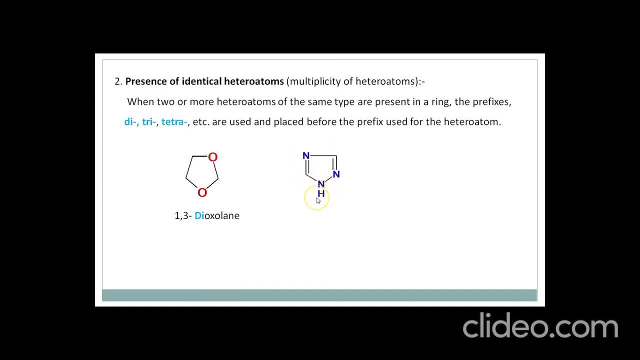 Now, here it is a five member unsaturated ring having how many nitrogen? One, two, three, So name is triazole, Triazole, Triazole, So it having a nitrogen, so aza, and it is, as it is, five member ring, we use ole. 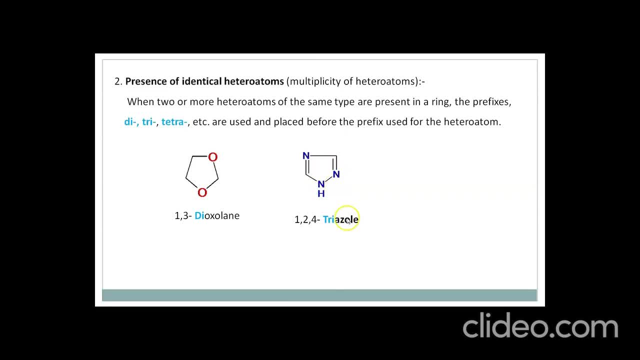 So name is azole, but as it contains the three nitrogen, we use prefix tri. So the position is one, two, three, four. So one, two, four, triazole. Now here is the next one. It is a example in which name is diazine, one, three, diazine, and the common name is: 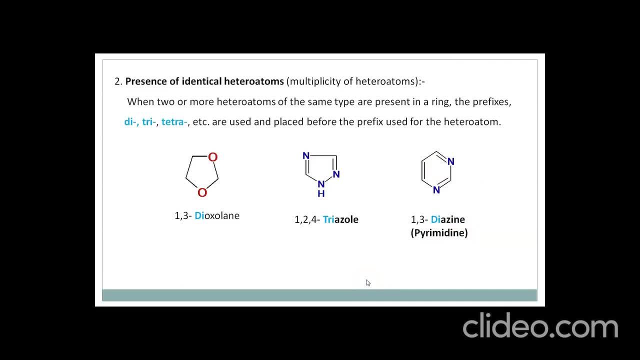 pyrimidine. So this is the second point In which we have seen the name for the heterocyclic ring and if it having a two identical heteroatom, then how to give the name for this. Now, moving to the next point, Suppose there are the two different heteroatoms are present, then what to do? 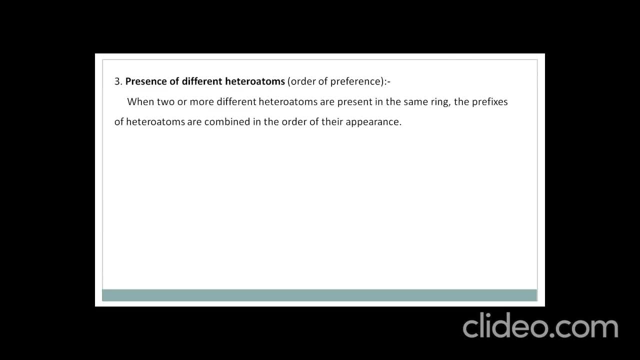 So in that case, when two or more different heteroatoms are present in the same ring, the prefixes of heteroatoms are present. So the prefixes of heteroatoms are combined in order of their appearance, Like we have seen, the prefixes in preferential order, like the first preference is given to. 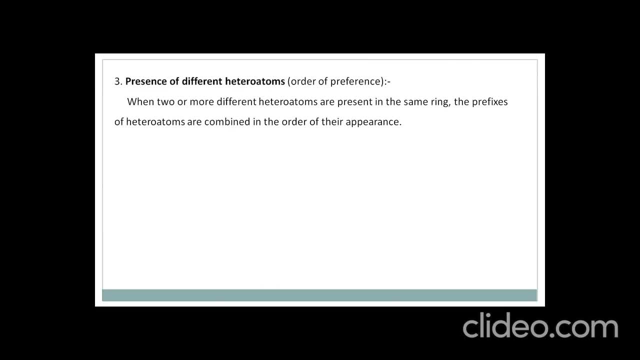 oxygen, then for sulfur oxygen, oxa sulfur, sulfur, thia, and for nitrogen aza. So you have to remember O S N, which is the preferential order. Here is the example: In nitrogen aza. So you have to remember O S N, which is the preferential order. 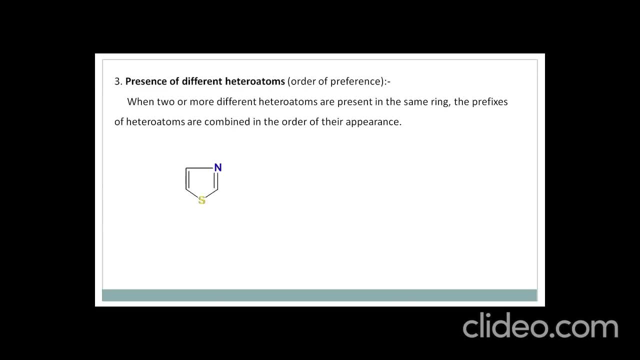 Here is the example: In nitrogen aza. So here it is common term in which it having a five members unsaturated ring containing sulfur and nitrogen. So in that case we give the preference to sulfur. so first of all for sulfur we use thia. 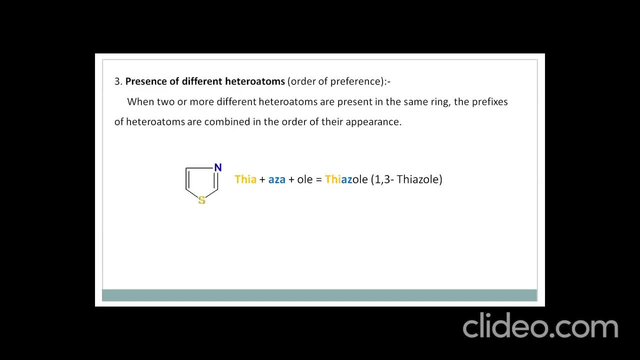 for nitrogen aza and as it is five members ring, we use stem ole. So combined it is thiazole. Ok, This is thiazole Here. weBUY AND ORDER the above sample Now last. please listen, it is possible, It will come here. 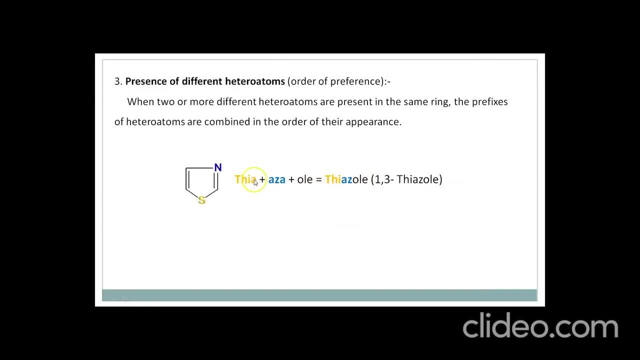 this a letter we drop, and also this a letter we drop because in both the it starts with the vowel, so the name is thiazole and as we give the preference to sulfur, so it having a number one, so one, two, three. this point we discuss. later on let's see the second example, in which it having oxygen. 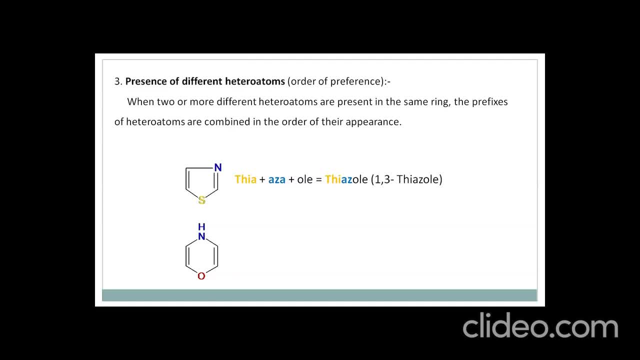 and nitrogen heteroatom, so which one having preference obvious to the oxygen. so write the prefix firstly for oxygen as oxa, then for nitrogen as a, and as it is six member ring, the stem we use is ine, so commonly the name is oxazine and it is a one for oxazine. 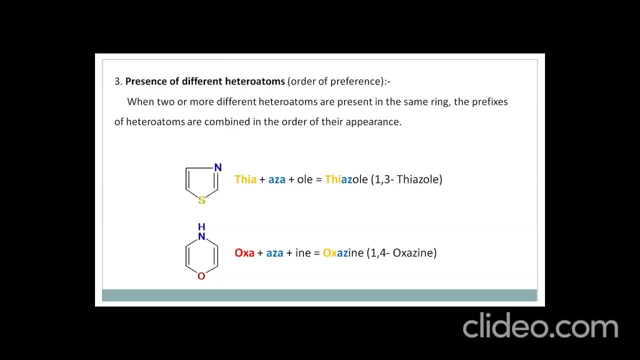 so this is the applicable or we use this when it having a presence of different heteroatoms in a ring. now next point is numbering. so if it having one heteroatom, then the numbering in in the ring starts from the heteroatom and giving the position and proceeds in such a way that 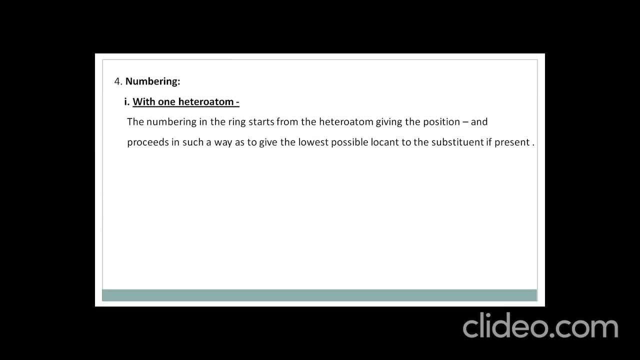 as to give the lowest possible locon to the substitute if it have like. here is, just take example, it a ring having nitrogen heteroatom. so we give the numbering from the nitrogen. so first to the nitrogen, accordingly you have to give aば. so first is to the nitrogen, then accordingly to give a number. now, second example: this is the Pieridin. now second example. in that case it is the Patrick Chiang in the second example. in that case it is the Pieridin now. in that case it is a Piridin ring, but it having a substitute and we give number of variation of rivers. 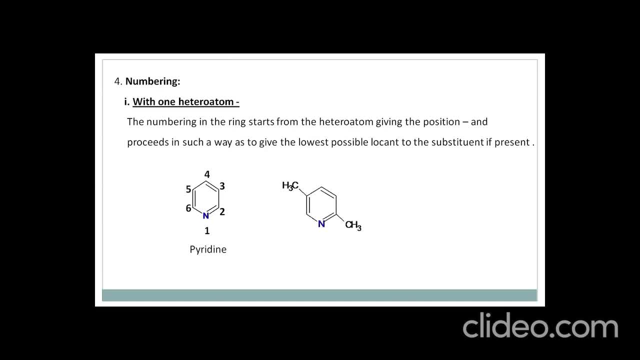 only in this case it is a second one in the trying. first. c ought be to continue with the a pyridine ring, but it having a substituent. so from where obvious, you have to give the number one to this nitrogen and where to give second number, whether to the clockwise, whether to the 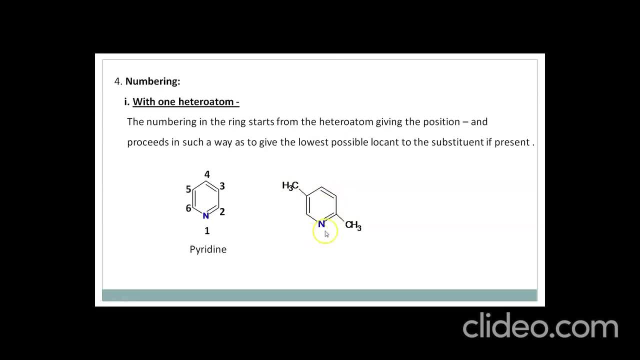 clockwise or anti-clockwise manner, so you have to choose. you have to give the lowest locant to the substituent, okay. so if you give from this, then it is having second, so it is a preferable. so one, then two, three, four, five, six. so name for this is 2, 5 dimethyl pyridine. 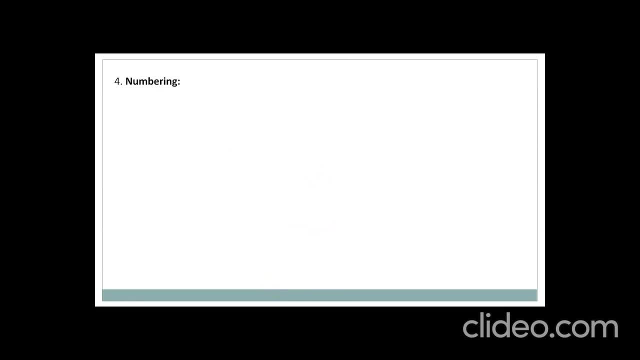 getting now. next is with two or more identical heteroatoms, if the ring it have. when two or more identical heteroatoms are present in a ring, the ring is numbered in such a way that the heteroatoms are assigned the lowest possible set of number locants. now here is 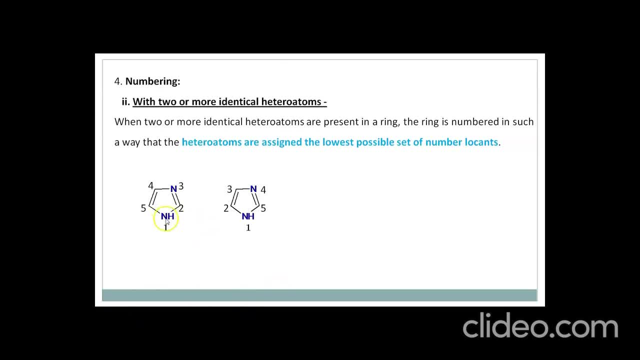 the example. so you, if you see this. so the first is given to the heteroatom and accordingly you have to give the numbering but to this it having a lowest possible set of number locants. so the lowest possible set of number to the another heteroatom. so here is the preferable one. two, three, 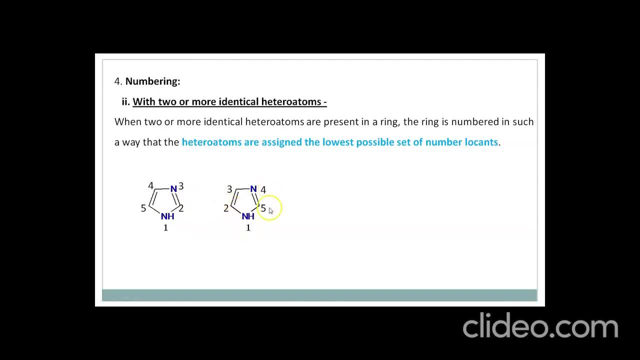 and here is the one: two, three, four, five. so we have given the number. so which one is correct? so in case of first it having a one, three number given to the heteroatom, and in this set the one, four number is given to heteroatom. so which one is correct? one. so obviously the first one is correct. 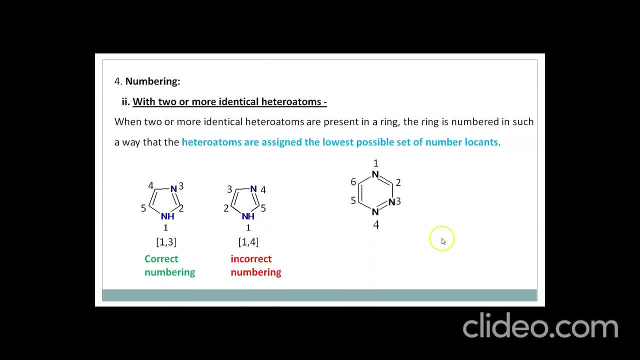 and this is incorrect. now take another example. here is the. the numbering is given. suppose i given as to this nitrogen one, then two, three, four. and if also i give this one, two, three, four, so if i give the numbering to this, then the heteroatom having a one, three, four numbering and in this set it having one, two, four. 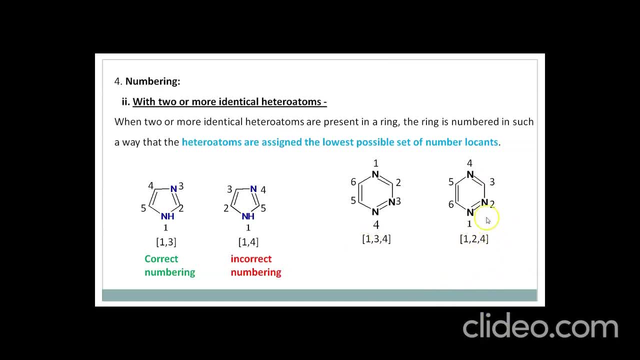 so from that which one is correct, obvious, this one is correct and this is incorrect numbering. so remember this: when two or more identical heteroatoms are present, then you have to give the numbering in such a way that the heteroatoms are assigned the lowest possible set of number locants, now the if it having two or 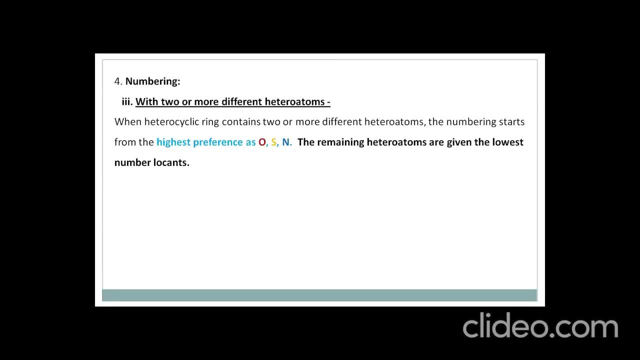 more different heteroatoms. when heterocyclic ring contains two or more different heteroatoms, the numbering starts from the highest value. 2 or more different heteroatoms would have less numbering. the numbering starts from the highest preference as Oxygen, Sulphur Nitrogen. 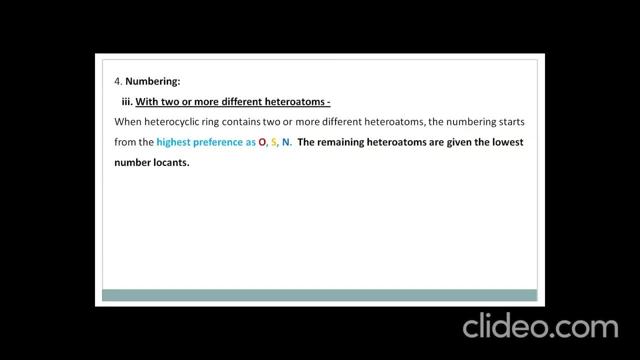 The remaining heteroatoms are given the lowest number Locant. Just take example: here is the heterocyclic ring which having a two different heteroatoms, So preference is to the Sulphur. So put the first number to Sulphur and then 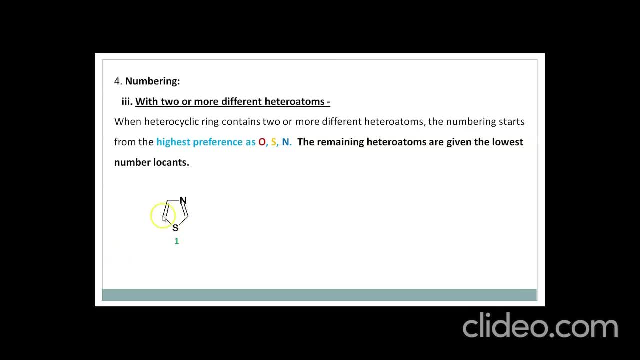 where to give second number, whether to this or to this Carbon, So obvious. to this Carbon, because if you give this second, then this Nitrogen having lowest Locant. So 2, 3, 4, 5.. This is the 1, 3 Thiazole. 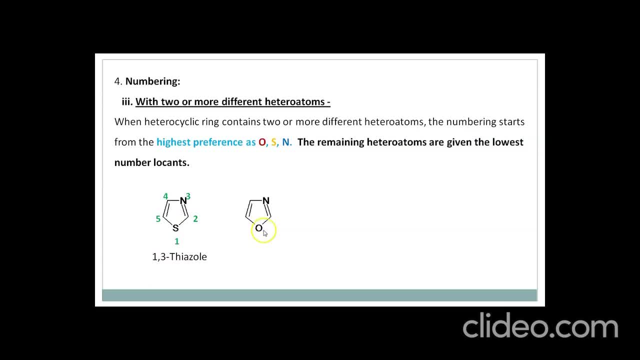 Here is the another example: and we give the first number first priority to Oxygen, Then to lowest is to the second heteroatom, So 1, then 2,, 3,, 4,, 5, and it is the Oxazole, and give the position of this. 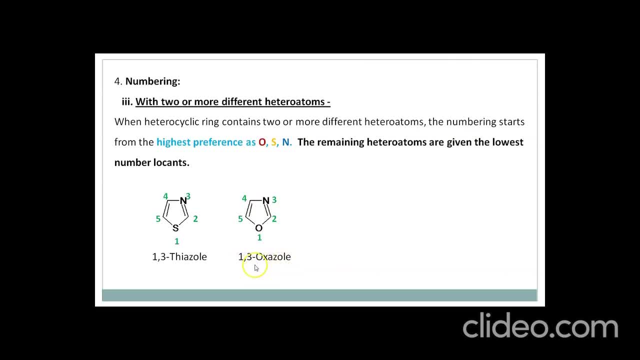 So we have to put number 1, 3, Oxazole, So indicate at first and third position the heteroatoms are present, and first to the Oxygen and third to the Nitrogen. Then here is the another example, and which is the 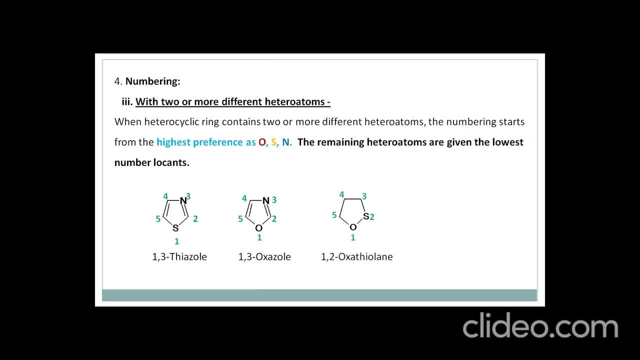 numbering and name is Oxathiolone, and here is the numbering: 1.. Obvious, we put the second to this Nitrogen, not 2 here, because if you give the 2 number here then it having a highest number, But if you put the second number then it having a lowest number. Locants: 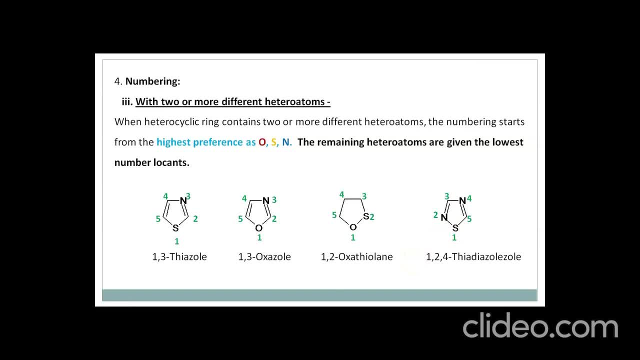 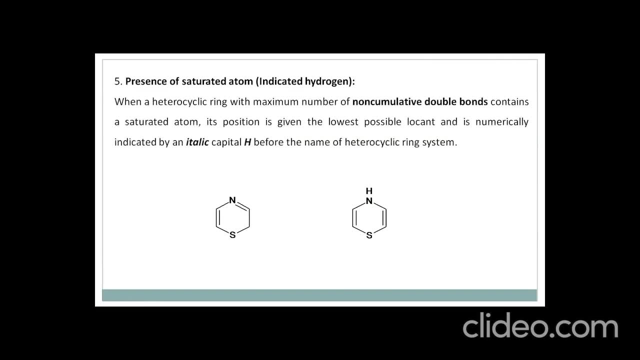 So name is the 1,, 2,, 4 Thiadiazole. Now here is the next- is presence of saturated atom, which can be indicated Hydrogen. So when a heterocyclic ring with maximum number of non-cumulative double bonds. 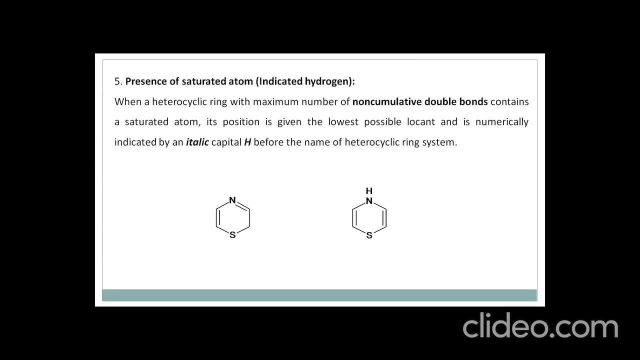 contains a saturated atom, its position is given the lowest possible Locant and is numerically indicated by a italic capital H before the name of heterocyclic ring system. So here is the example. Like in this ring, the Sulphur and Nitrogen heteroatoms are present. 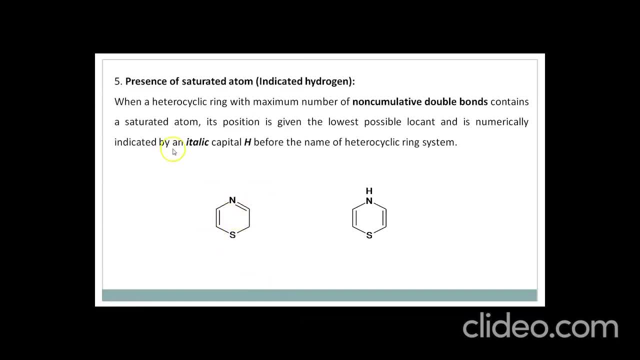 and we have seen the previous rules for this. So you have to put first number to this Sulphur and as it contains a, it is unsaturated ring but it is a non-cumulative- double bonds are present. So here is the more Hydrogens are present. 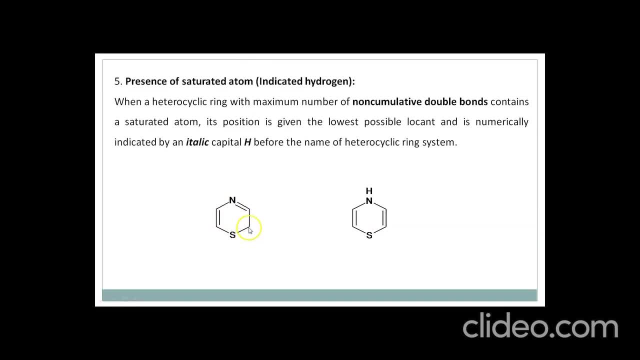 Here is the CH2.. So you have to give the second position to this Carbon. So 1st, 2nd, 3rd, 4th, 5th, 6th, So to the second position, the Hydrogen is present. 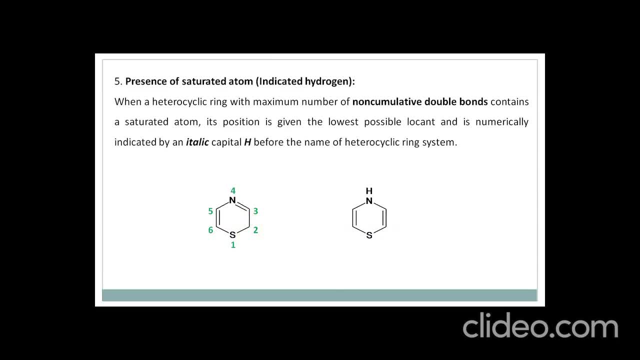 So you have to give written it in italic and give the number. So it is 2H, 1 for Thiazine. Same the case for here to this Nitrogen, it having a Hydrogen, and the numbering is obvious: 1,, 2,, 3,, 4..